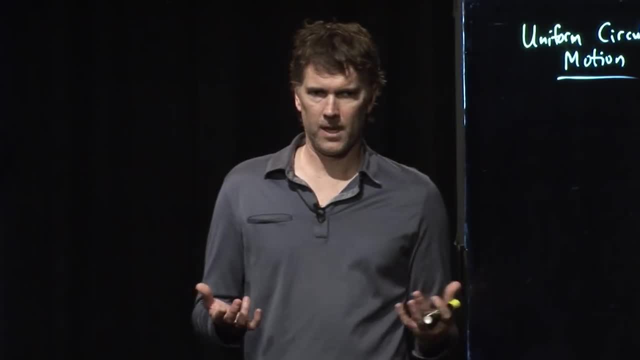 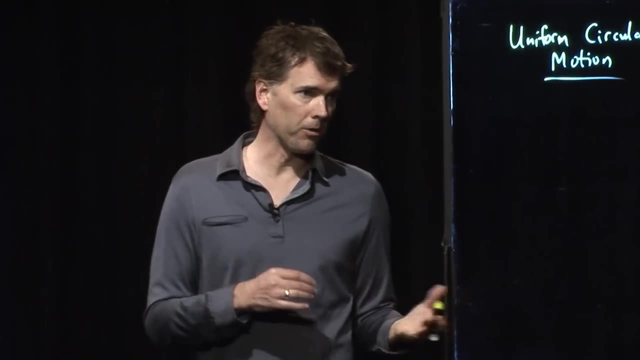 we're accelerating And that's because the Earth is pretty big. Okay, The Earth is pretty big And for its size, it's not spinning around that fast. Right, We're actually moving about a thousand miles per hour right now, But for the size of 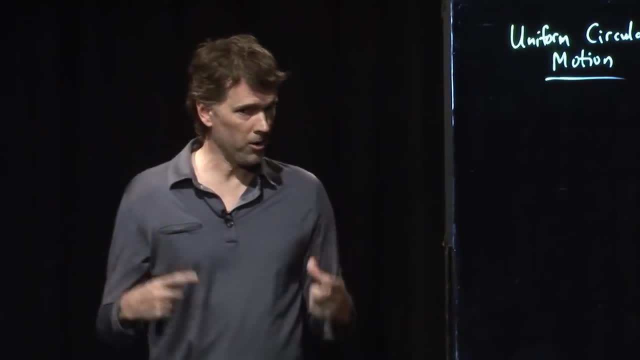 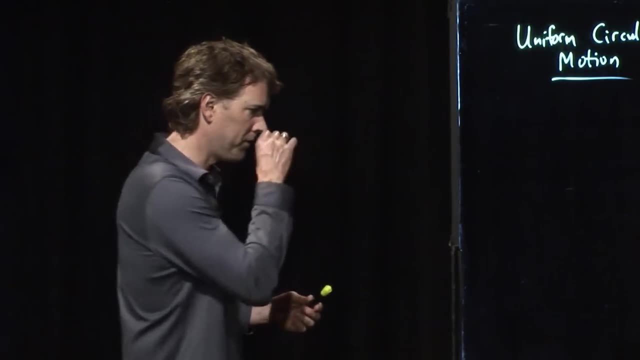 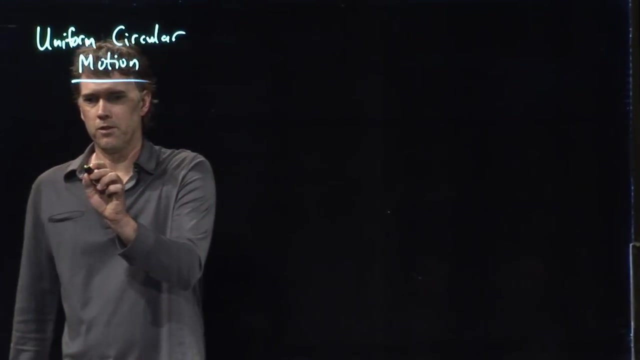 the Earth. that's not that fast. When you get on a small merry-go-round and you spin around on a merry-go-round, you definitely feel that acceleration All right, So let's talk about uniform circular motion. Okay, Uniform circular motion is just this. 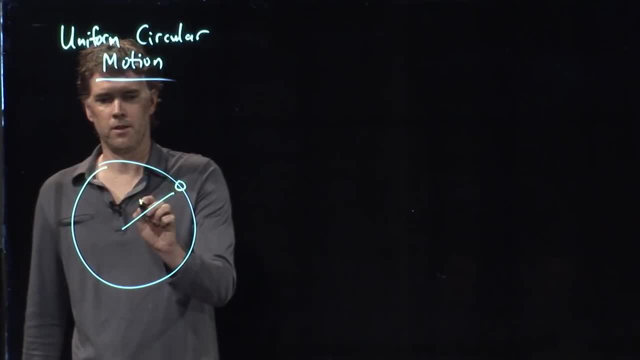 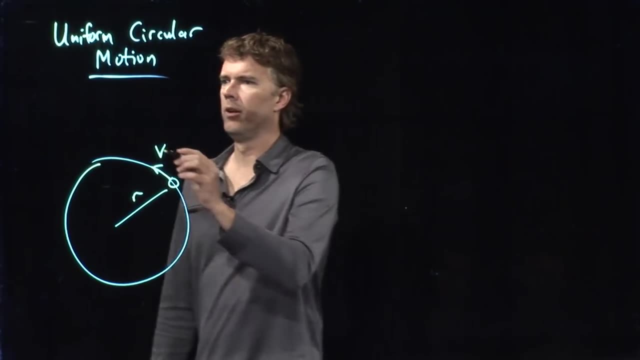 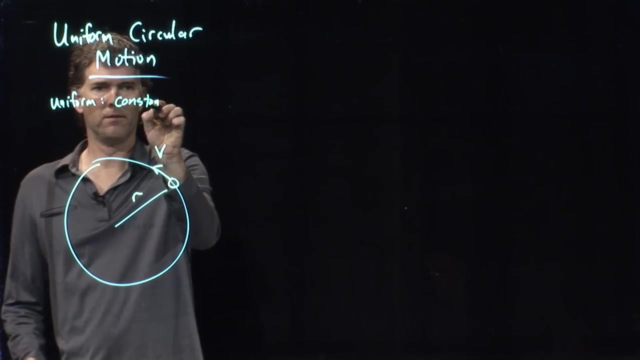 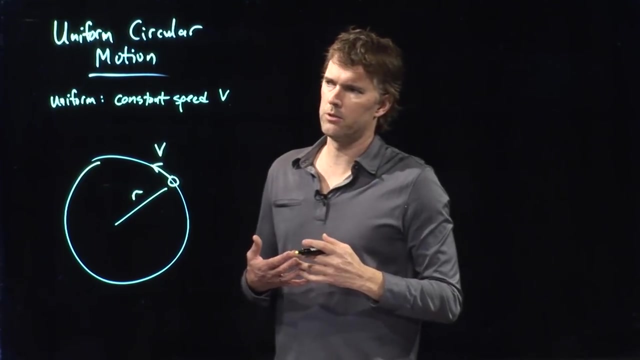 Something is moving in a circle of radius r and it's moving at a speed v. Uniform means constant speed. Okay, Later we will learn about non-uniform circular motion, which just means that the speed changes as you go around. But for now, let's just consider: 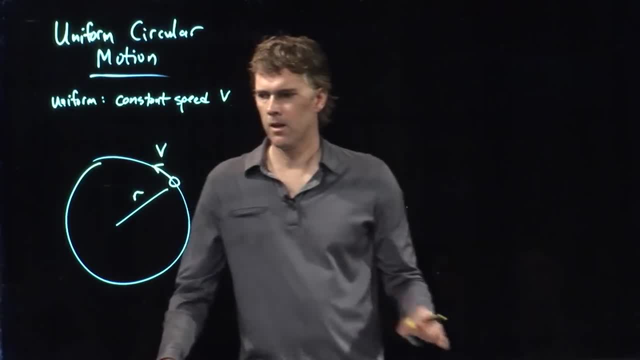 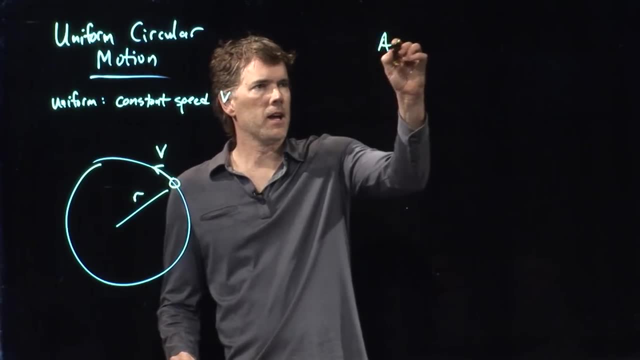 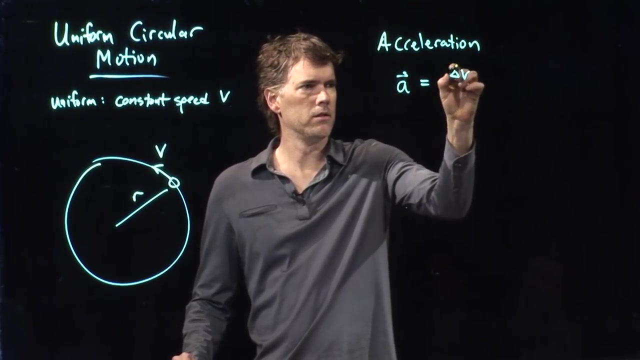 uniform circular motion, which is constant speed. Okay, That's what our picture looks like. We just said that we think we are accelerating, And we can probably convince ourselves pretty quickly that that is true, because acceleration is delta v over delta t, And delta v is the change. 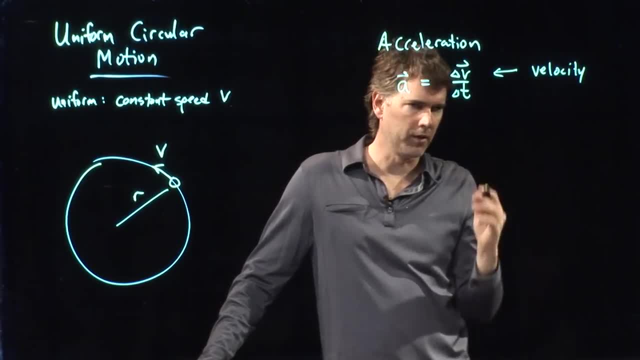 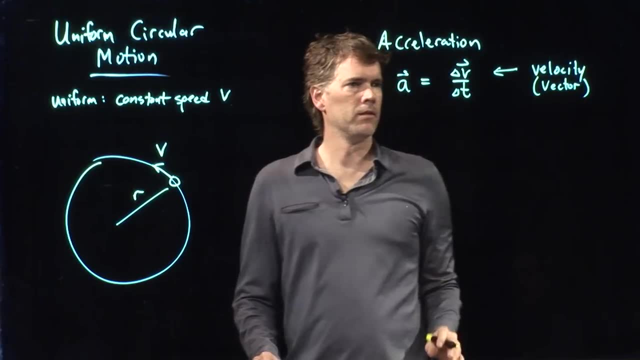 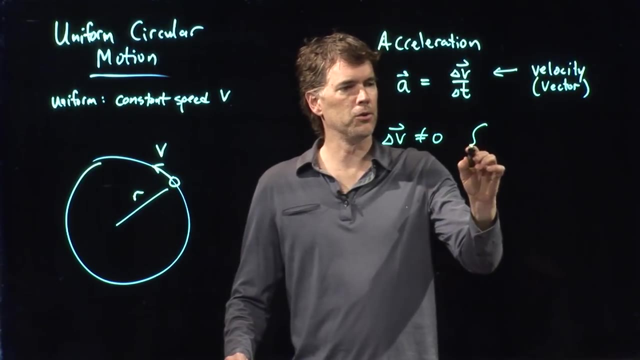 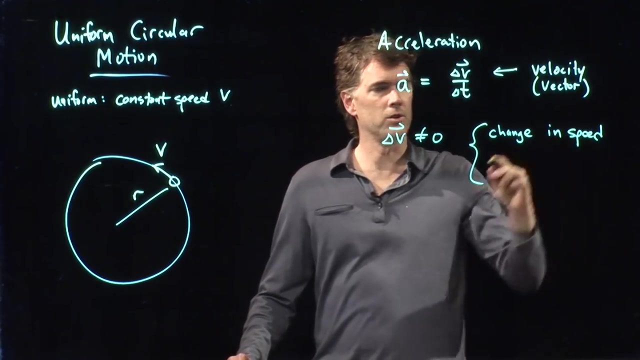 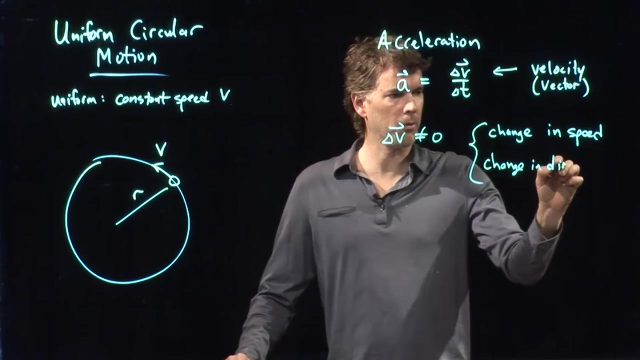 in velocity. It's velocity of vector or scalar. It's a vector. So if you have a delta v that's nonzero. that could be due to change in speed, which is the magnitude of velocity, or it could be change in direction. Okay, When you're. 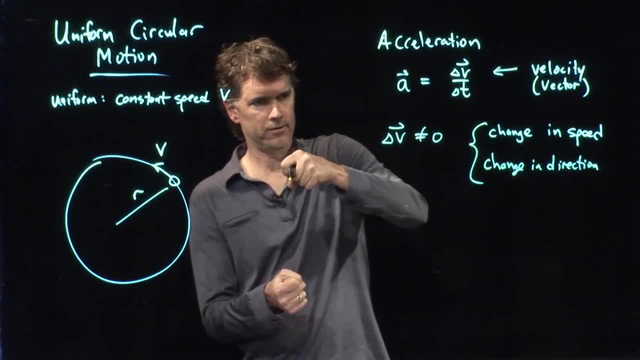 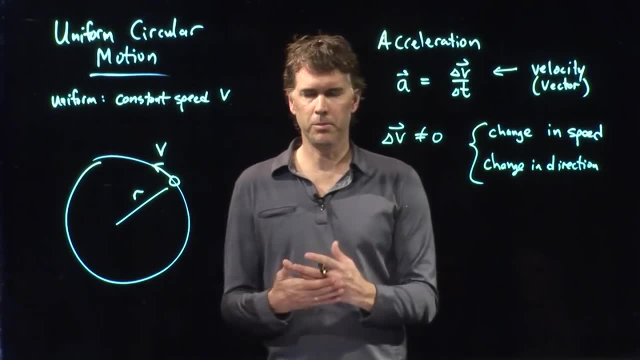 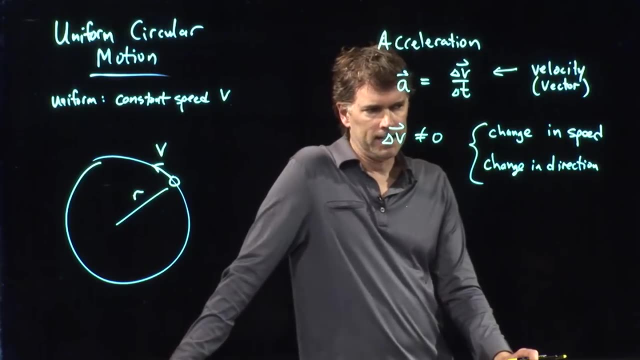 driving down the road and you turn your wheel to the left, you feel that acceleration because you're changing the direction of your car. You're not changing the speed of your car, especially if you don't hit the brakes, You're just changing the direction. okay, So how does this? 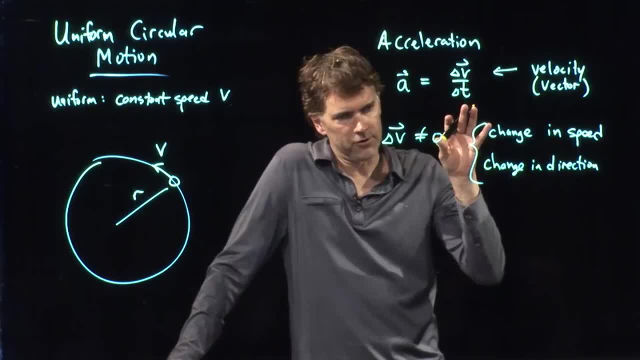 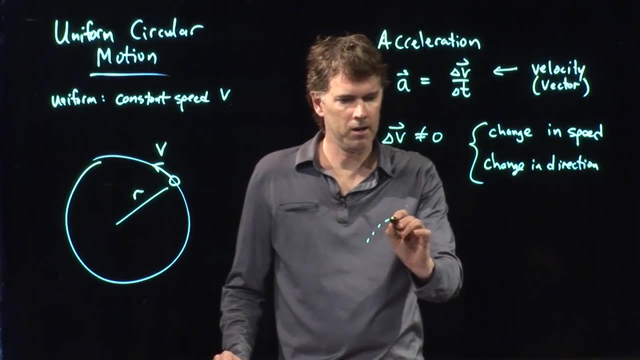 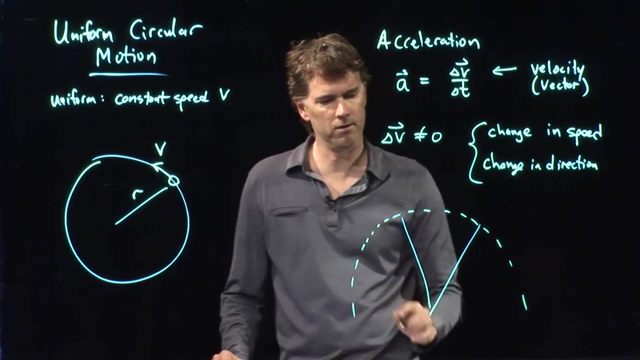 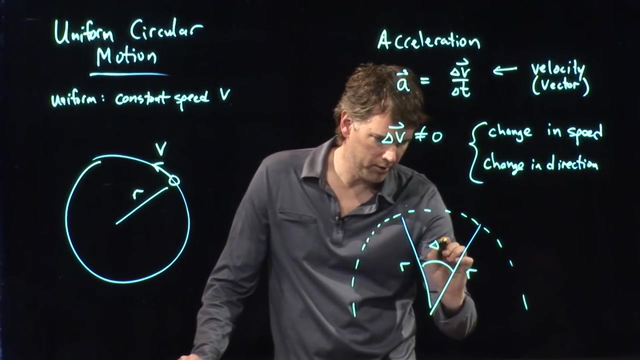 lead to an acceleration. How does changing the direction lead to an acceleration? Well, the way we're going to visualize it is the following: Here's a section of our circle, Here is a radius, vector r, and we're going to identify this angle that you traverse. 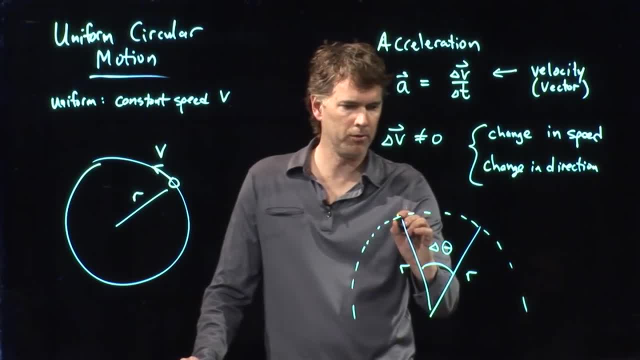 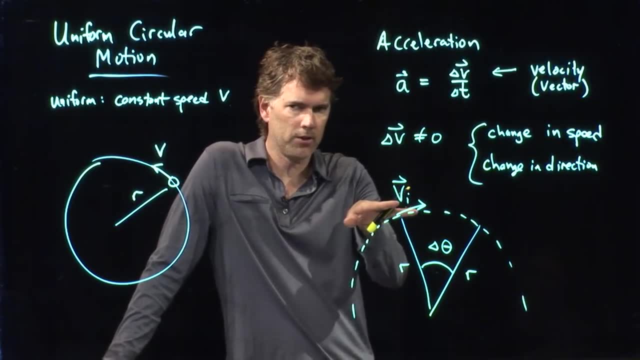 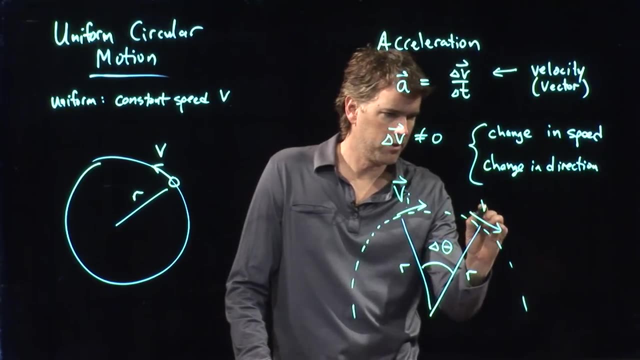 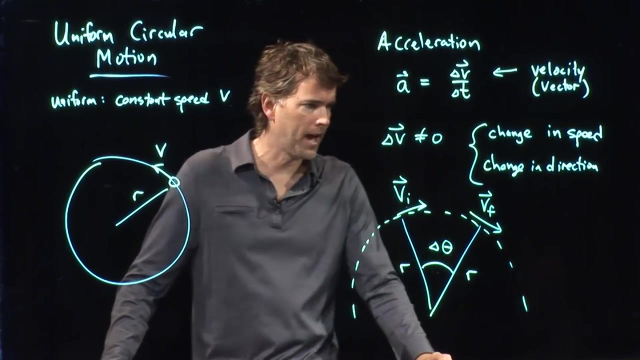 as delta, theta, and let's say that we're moving in this direction. okay, Your velocity is always tangential to the circle in uniform circular motion. So the initial velocity is there, the final velocity is there. We have clearly changed directions for our velocity, and so that is going to lead to an 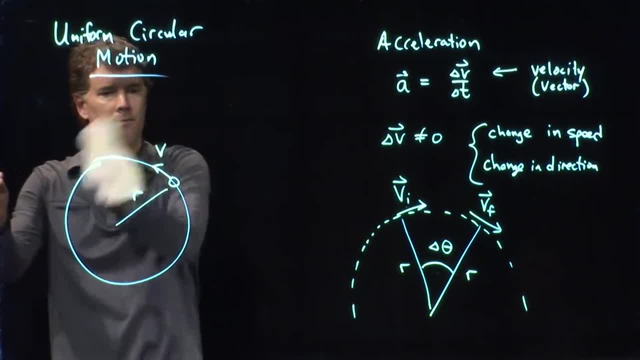 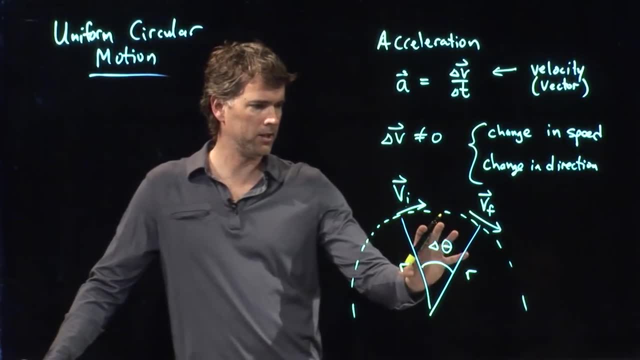 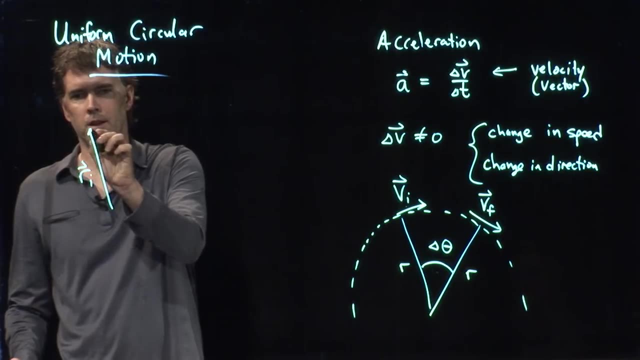 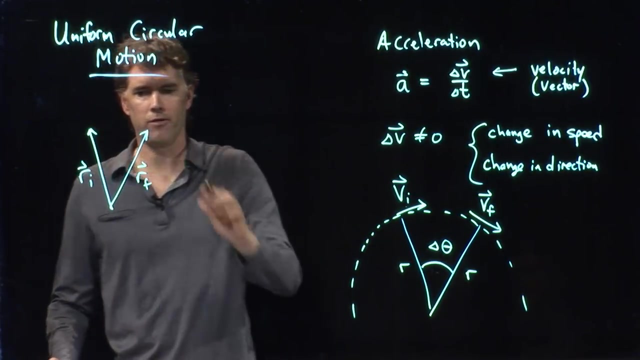 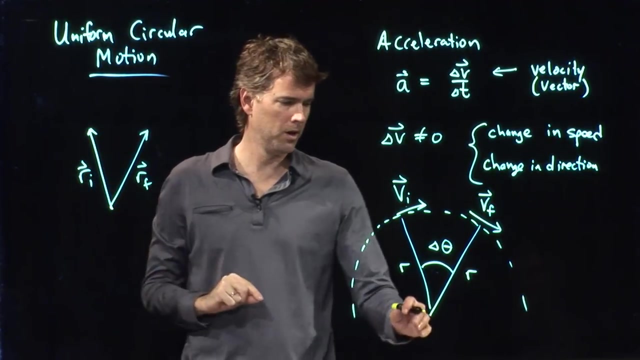 acceleration, Okay. so let's take a look at this picture in a little more detail. right, Where did I start? I started at a position. there r initial. I ended at a position, there r final, Okay, vectors for position. they always define relative to some origin. We'll make the origin the center of the. 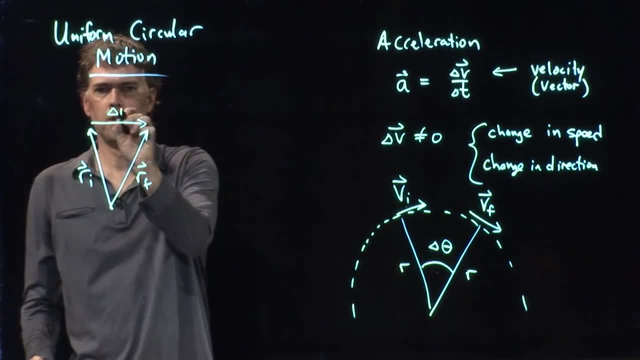 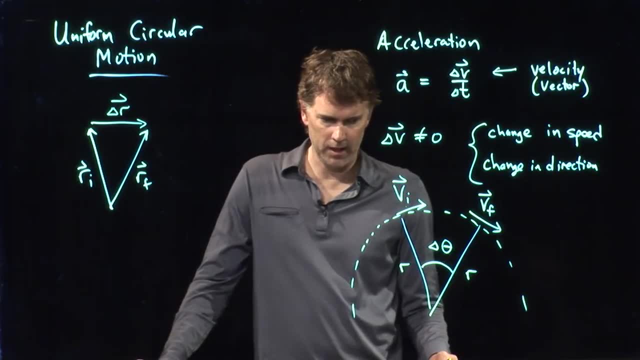 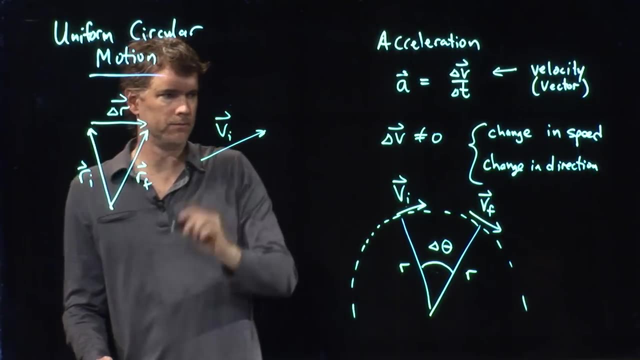 circle. The difference between those two is, of course, right there, okay, So what about the velocity vectors? Well, it looks like the velocity vector v i is up and to the right, but v f is down and to the right. 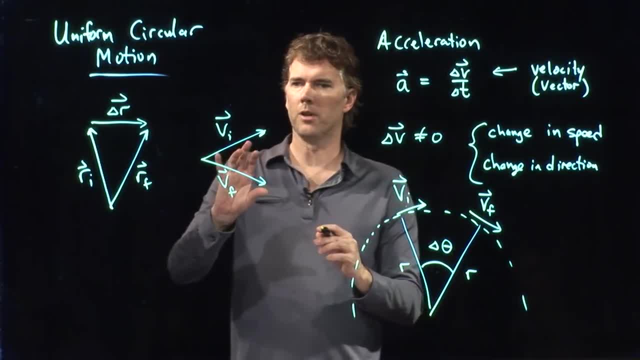 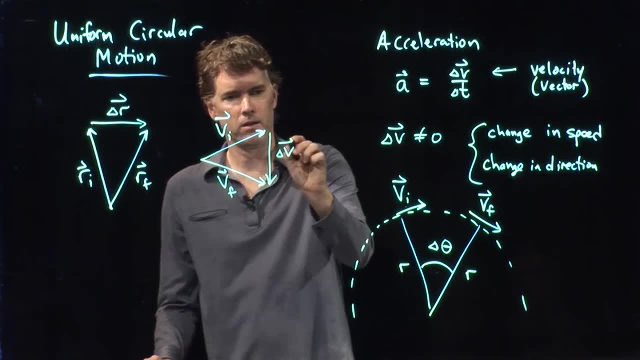 And if I do the difference of those two, remember, you can do your tip to tail approach by flipping the sign of one of them, but you can probably convince yourself pretty quickly that delta v is going to look like that. okay, I was going up, I've changed to going. 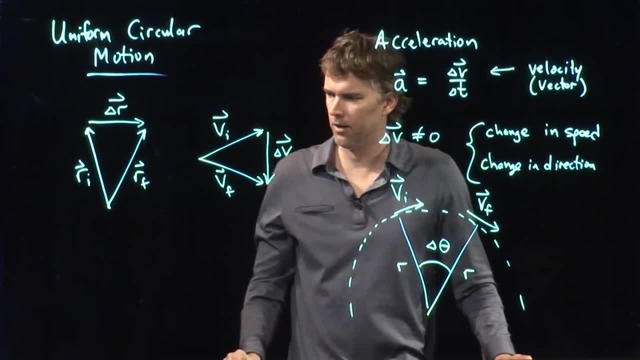 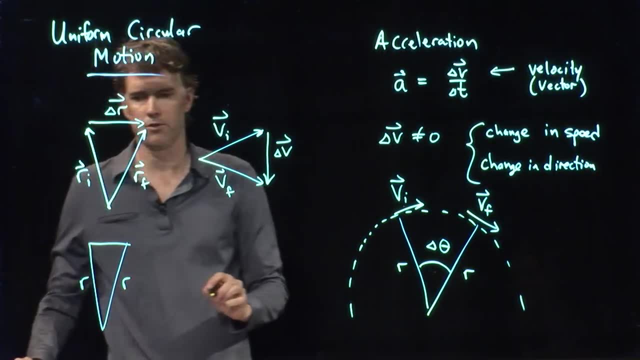 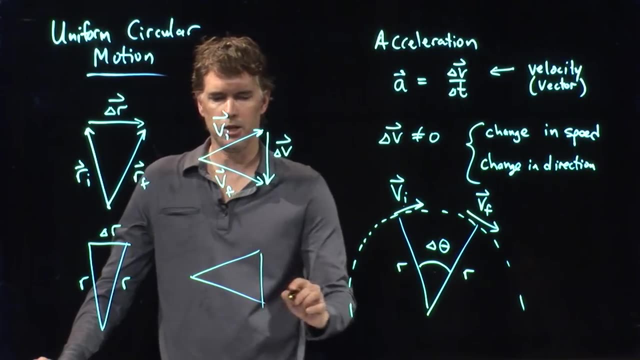 down, and so the delta V has to be pointing down. All right, but these are just magnitudes. now, The radius of the circle doesn't change. That side is just delta R. If we are in uniform motion, the speed doesn't change. 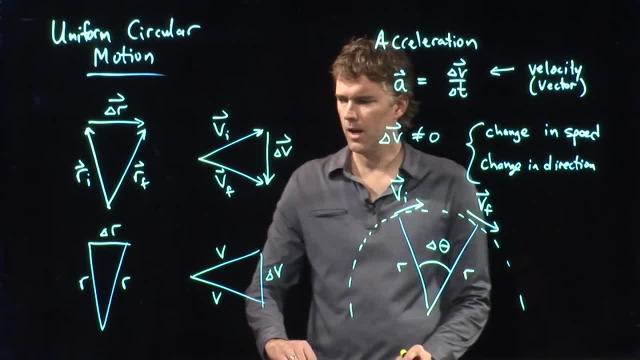 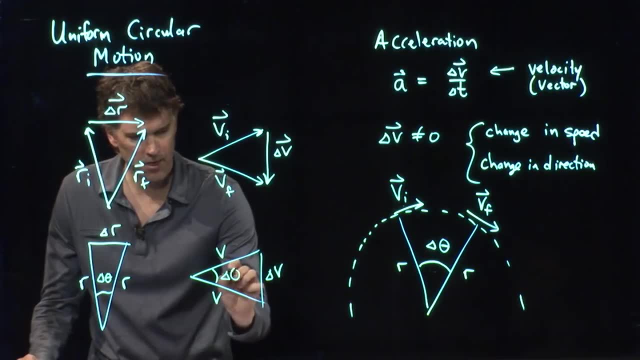 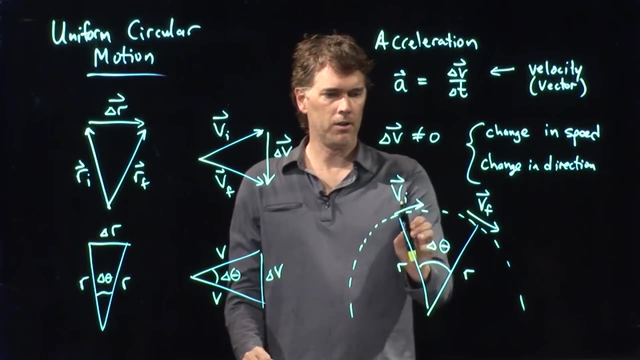 That side of the triangle is just delta V. Both of these are making an angle of delta theta. all right, This is the way we defined it. How do you see this? Well, this is always a right angle, and that's always a right angle. 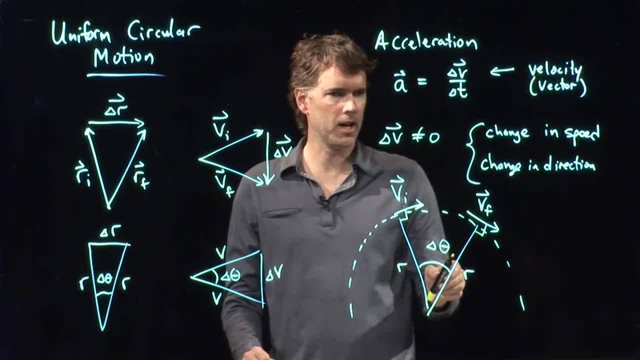 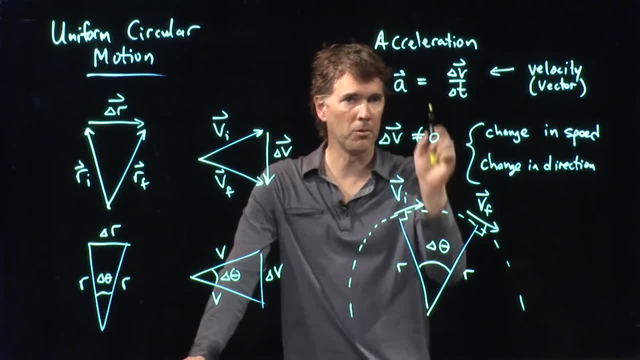 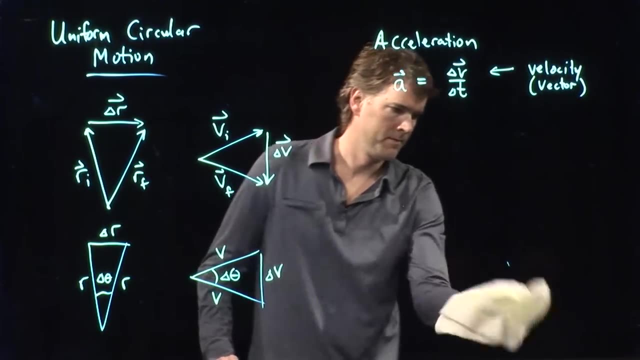 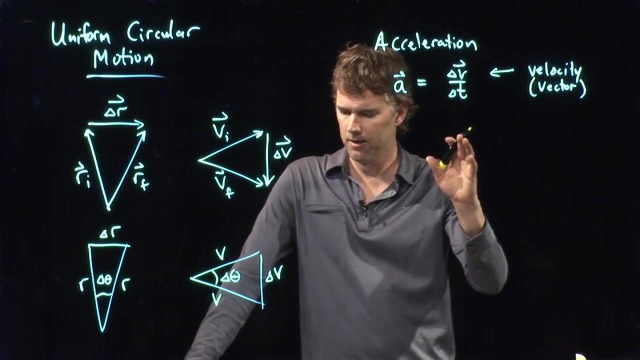 So if I add 90 degrees to VI and I add 90 degrees to VF, they both are going to traverse the same delta, theta. Okay, let's go back to our acceleration. We said that acceleration was delta V over delta T. but if I look at these pictures now, 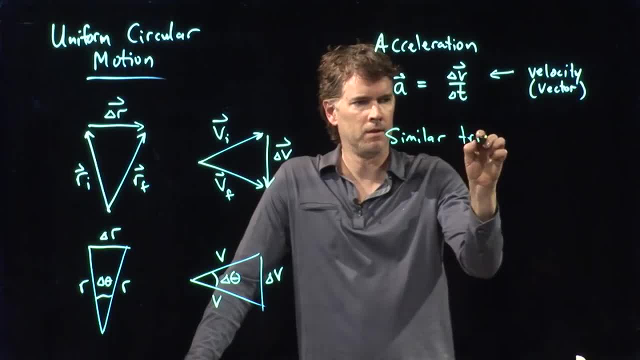 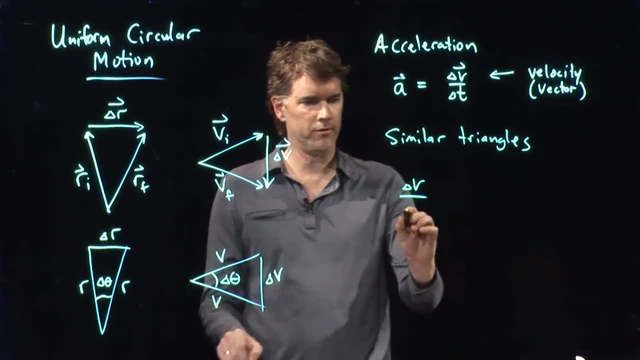 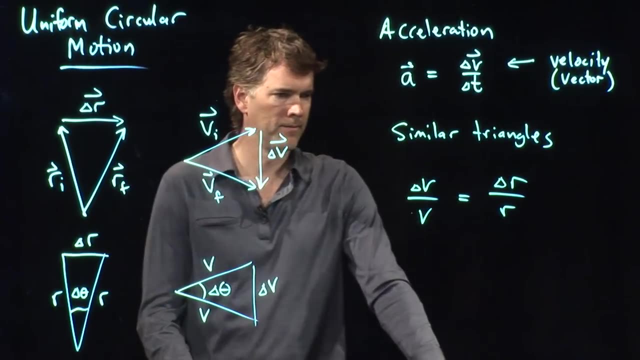 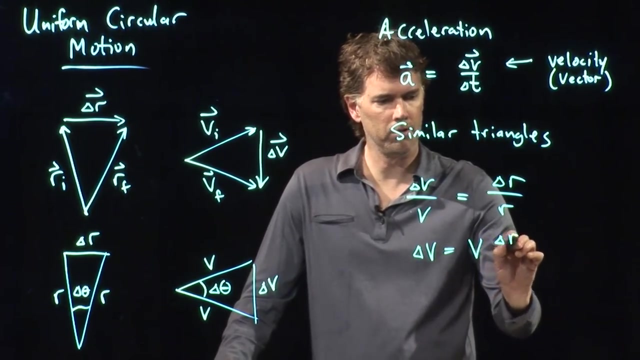 those triangles are similar. And if they are similar triangles, then I can write the following: Delta V over V is exactly the same as delta R over R. And now I can solve this for delta V, I get: delta V is equal to V times delta R over R. 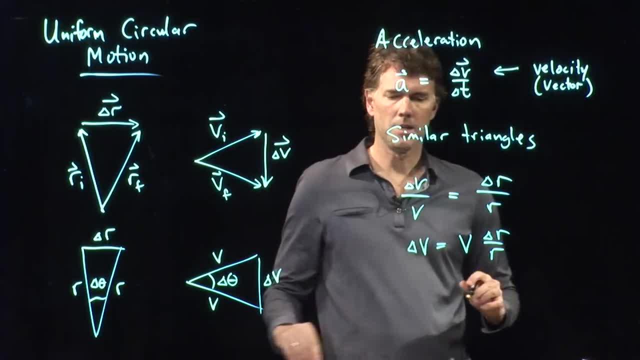 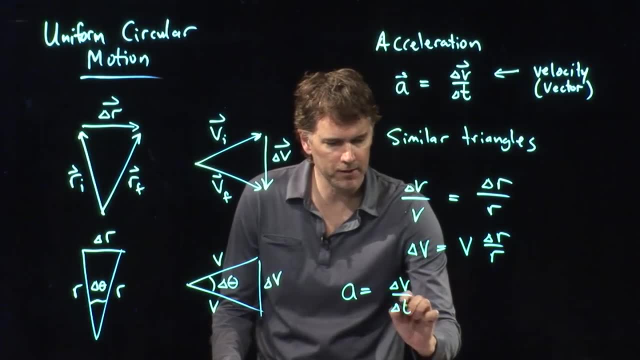 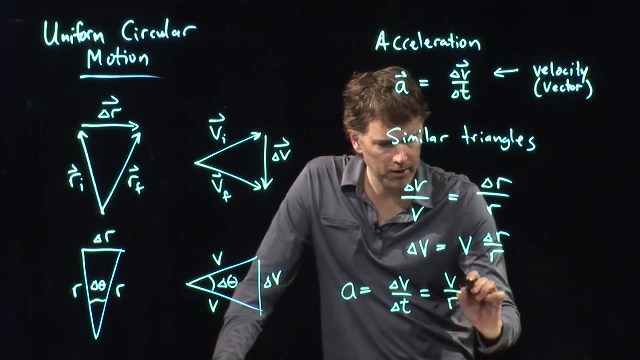 I just multiply it across by V, And now let's plug that into A: A. the magnitude of A, we said, was delta V over delta T, And here's my delta V, And so I can plug that in. I get V over R times, delta, R over delta T. 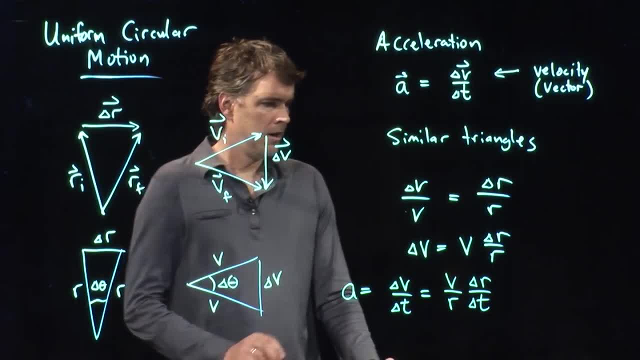 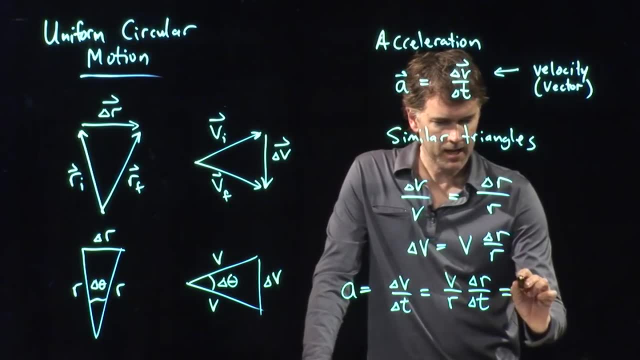 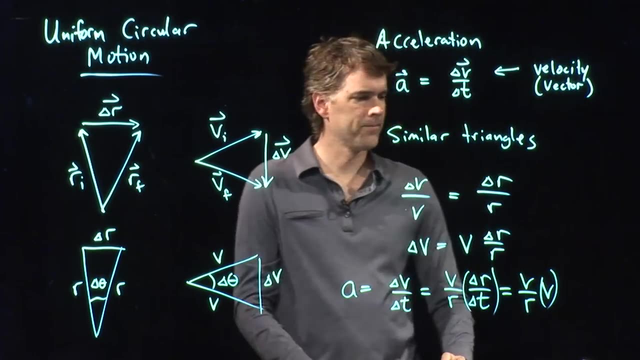 which I carried in. Okay, I can plug that in from there, But delta R over delta T, that's just how far you've gone in some amount of time, which is again just your speed. Delta R over delta T is just V. 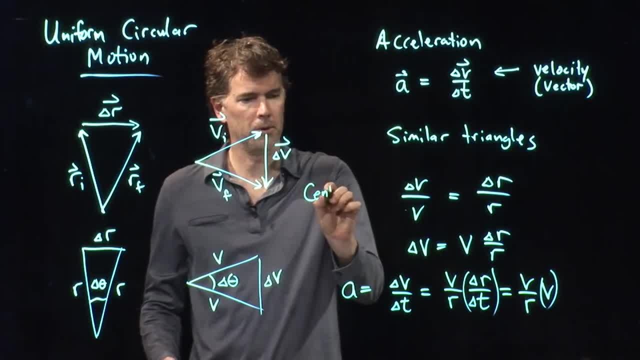 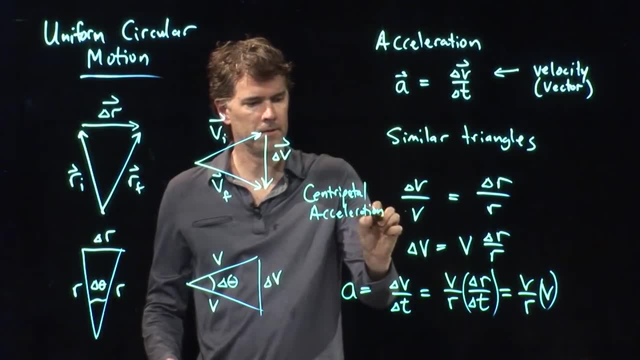 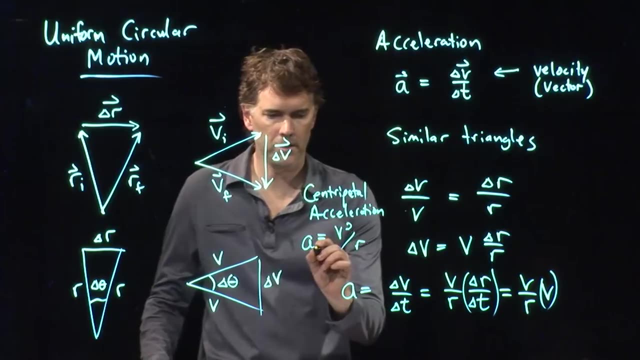 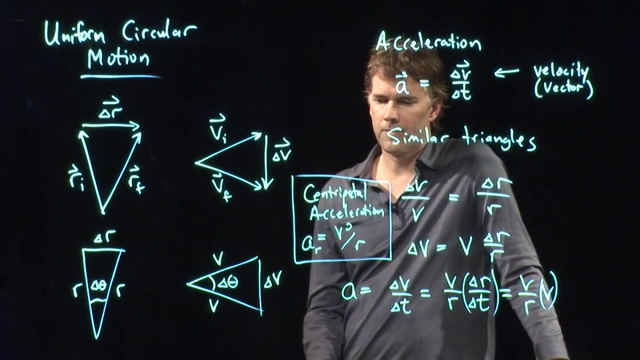 And so we get what we now call centripetal acceleration, And it is A equals V, A equals V squared over R, And we typically put a little subscript on it: either C or R. I like to use R for radial. Some people use C for centripetal. 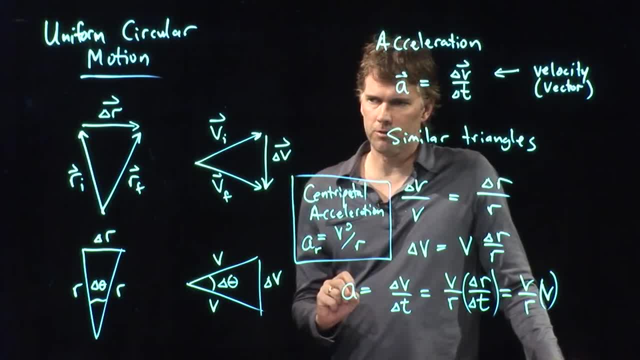 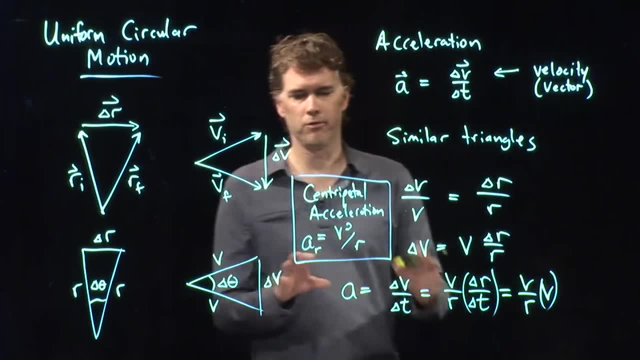 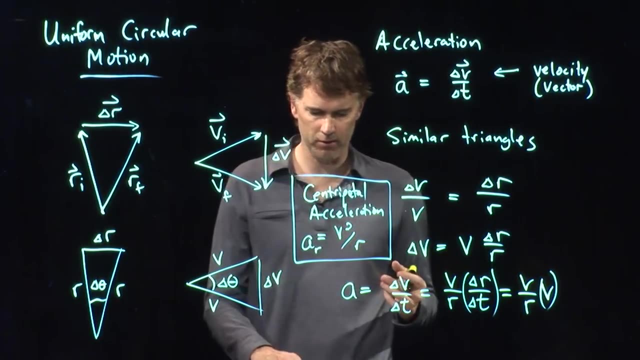 But what this means is, anytime you're moving in a circle, you have a centripetal acceleration towards the center of the circle which has this magnitude V squared over R. okay, That's how fast you are accelerating towards the center of the circle.